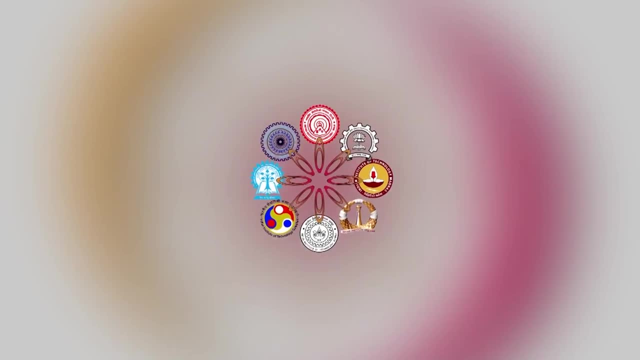 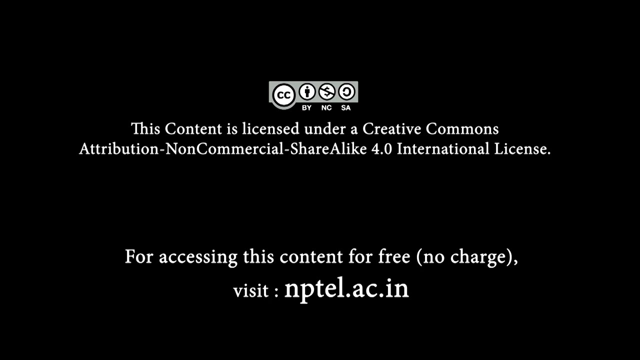 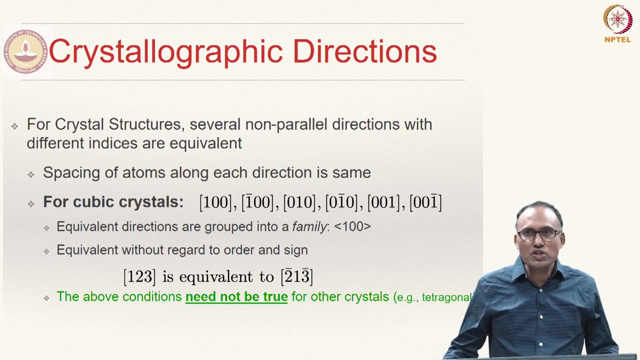 Welcome back. So in the last class we have discussed the crystallographic directions, particularly for cubic crystals, And then we have actually also introduced the concept of equivalent directions. So for instance, for a cubic crystal you have 1, 0, 0, 1 bar. 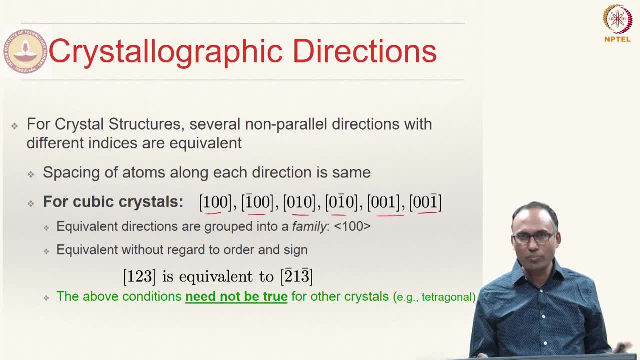 0, 0, 0, 1, 0, 0, 1 bar. 0, 0, 0, 1, 0, 0, 1 bar. All these are equivalent directions And these are called a family of equivalent directions, And the family of equivalent directions is: 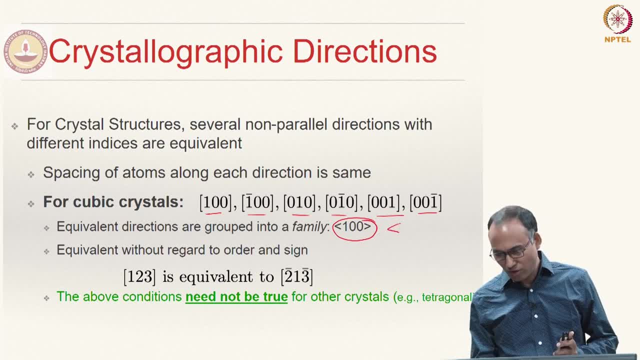 represented by this sort of a representation. You have a Macaulay sort of a bracket and then 1, 0, 0. And all these permutations of these three indices will give you the equivalent directions for cubic crystals. And this way of representing equivalent directions will only work for cubic crystals. For other, 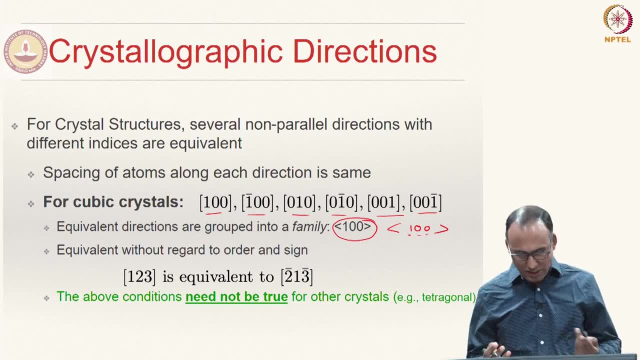 crystals, for instance tetragonal crystal. it may not work. It does not work. So this definition of equivalent crystals is what we are only…. You should keep it in mind that it is only right for cubic crystals, So, for instance, you can say that by that. 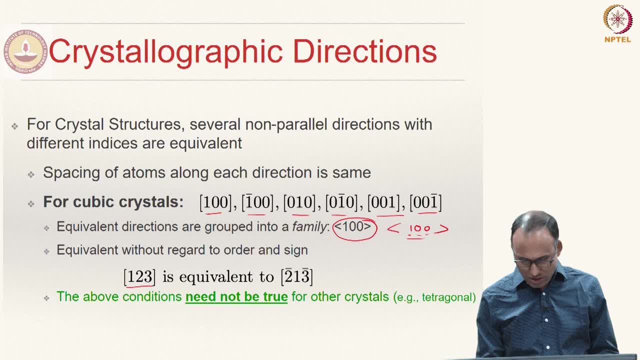 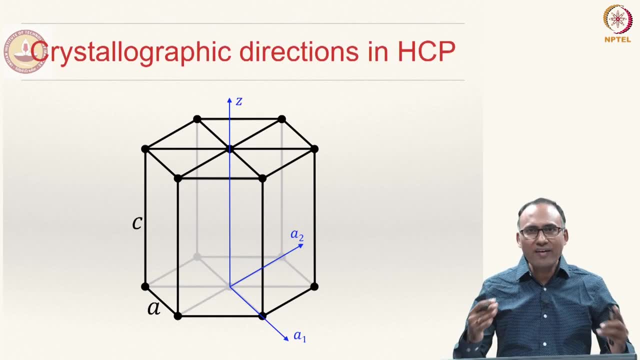 definition: 1, 2, 3 direction in a cubic crystal must be equal to 2 bar, 1- 3 bar, or 2: 1- 3 bar, And so on. So now, having discussed how the crystallographic directions are shown in a cubic crystal, now 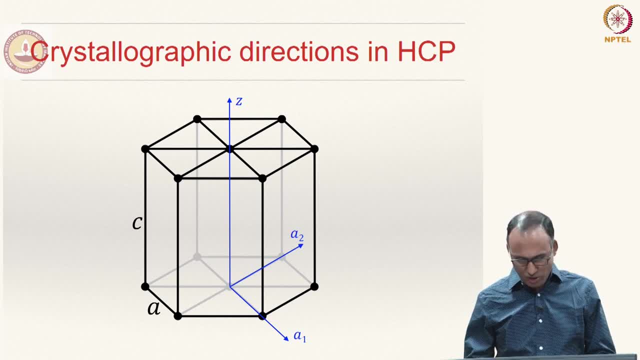 let us look at hexagonal closed pack structure. Suppose if we take a hexagonal crystal and which has 3 lattice vectors: A 1, A 2 and z. z is outer plane direction And in the base plane or basal plane you have these two lattice vectors A 1 and A 2.. 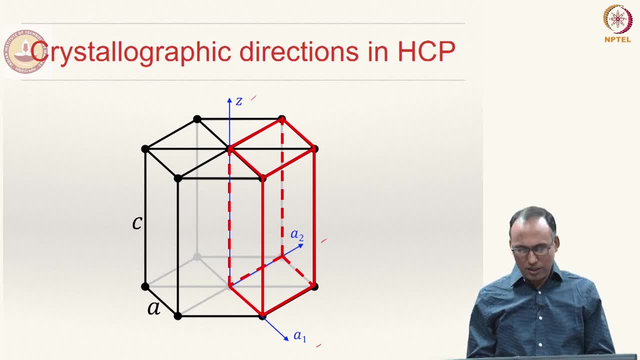 Alright, So this can also be our one of the definitions of our unit cell for a hexagonal closed pack system. And now let us look at this particular direction that is, the projection of this line, this guy, on to a 1 axis. a 1 vector is 0. that is why 0, 1 bar, because it is in the negative. 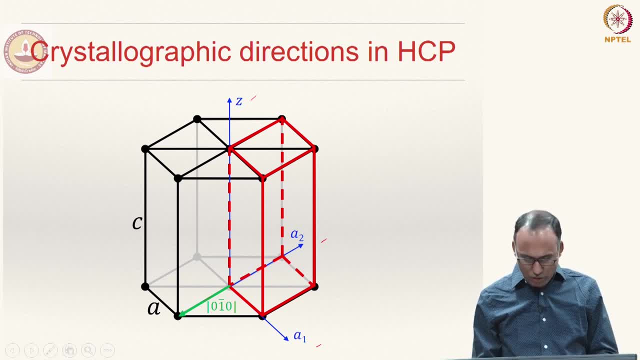 a 2 direction and the projection of this guy on to g axis is 0. So that is why this direction is 0, 1 bar 0, and then if you take this guy, again, 1 bar 0, 0, but if you take this direction, 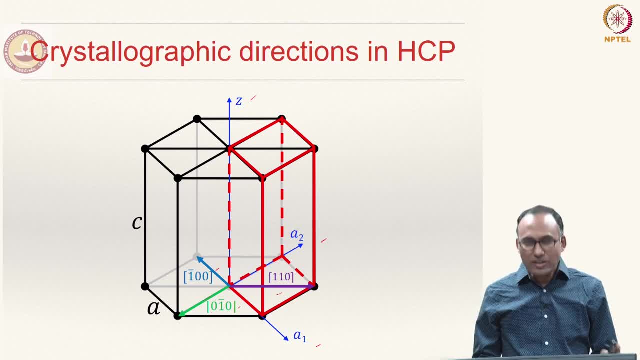 then you have 1, 1, 0 right. but you know that all the how do we say the equivalent direction? basically, when you are moving from this position by same amount, you should meet the another atom right by the same distance, by moving in the same distance. 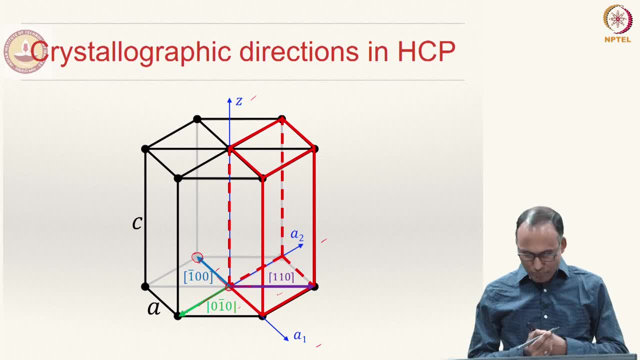 So here, this distance, this distance, This distance and this distance are the same. So by definition of our equivalent directions, these 3 should be equivalent directions. but when we are talking about the equivalent direction definition, as we have discussed in the cubic crystal, the indices, the miller indices, 1, the 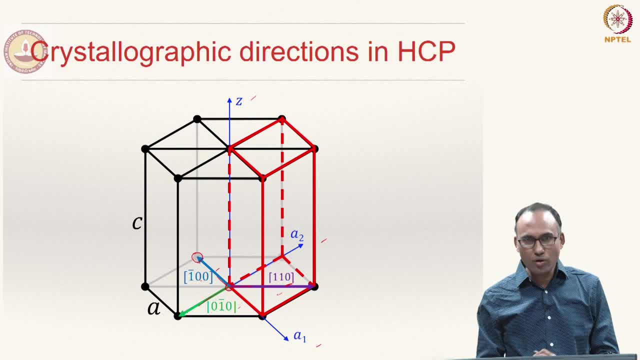 number should be the same. So you have 1: 0- 0. So you should have 2: 0s and 1 1s in any combination, but here you have 2 1s and 1 0s. 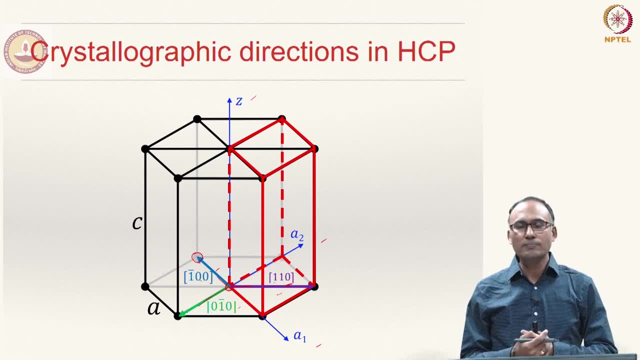 So if you have this, So this representation for crystallographic directions in hexagonal systems, you will not be able to use the permutation of same set of indices for representing equivalent directions, because the equivalent direction here, by looking at, you cannot say that these 2 are equivalent. 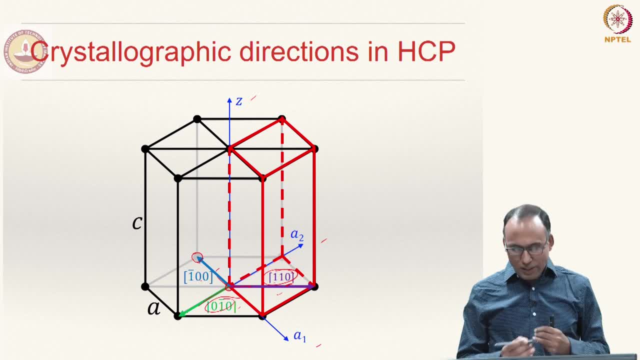 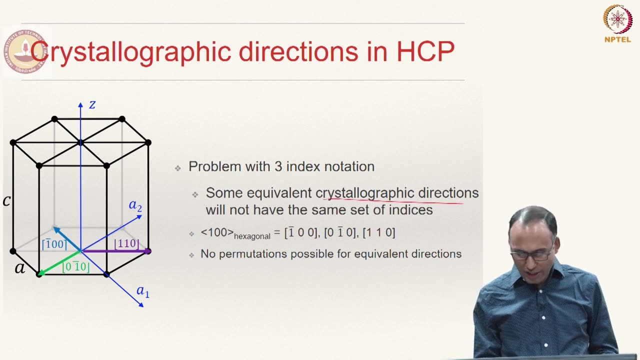 directions unless you actually draw and show that. So that is how the representation of that crystallographic directions is actually. the represented equivalent representation is actually breaking down. So this is the problem with three index notation, because some of the equivalent crystallographic directions will not have same set of indices, like these: 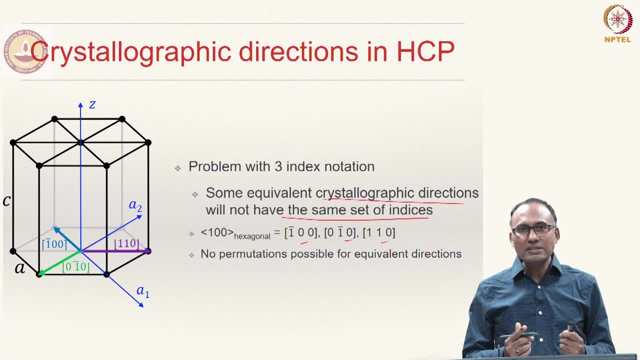 three. So that means the permutations are not possible for equivalent directions. if you are using such a definition: A 1,, A 2 and A 3, all right, So now, how do we circumvent this problem? How do we fix this problem? So the problem: 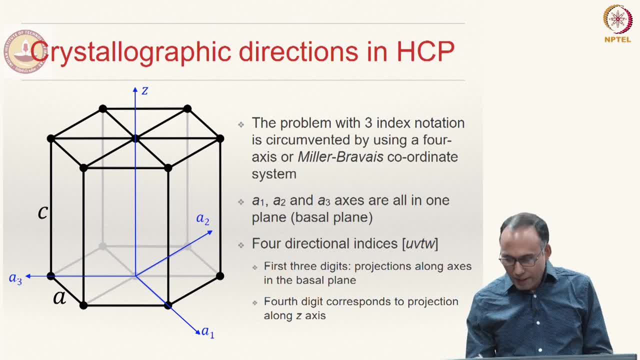 with the three index notation is usually is circumvented by a four axis or Miller-Grave coordinate system. So you have to do some modifications to your coordinate system. So instead of having three indices now you can have four axis system, So three axis previously. 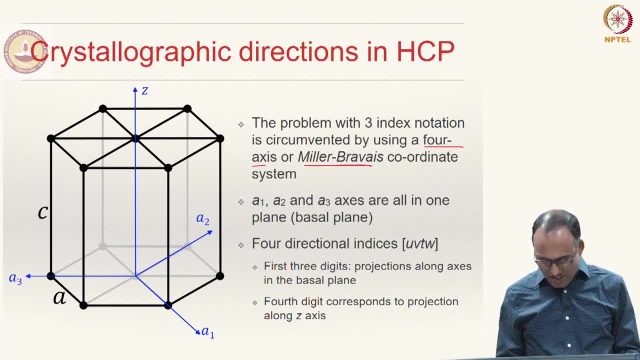 you have A 1,, A 2 and Z. Now we introduce another axis: A 1,, A 3,, A 4,, A 5,, A 6,, A 7,, A 8,, A 9,, A 10,, A 11,, A 12,, A 13,, A 14,, A 15,, A 16,, A 17,, A 18,, A 19,, A 20,, A 21,, A 21,. 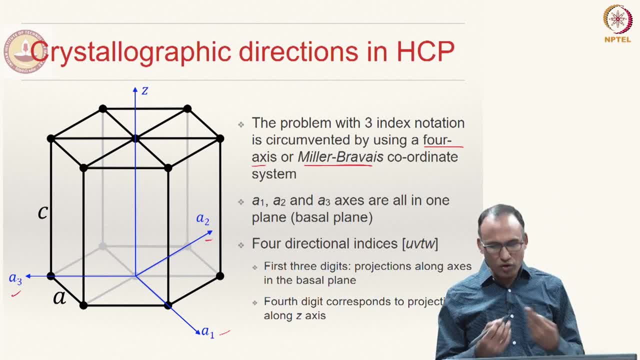 A 22,, A 23 and Z. So now you have four indices representation. So A 1, A 2, A 3 axis are in the basal plane and the fourth Z axis is the out of plane direction, that is in the 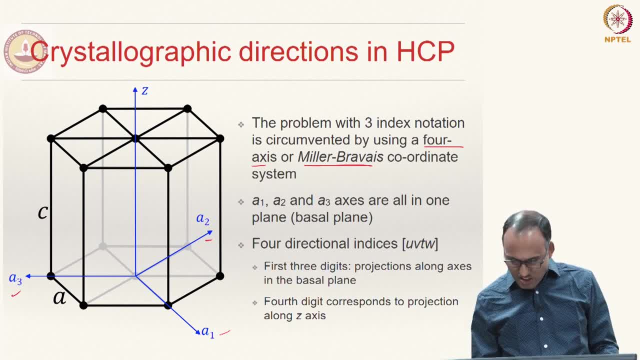 thickness or height direction. So the first three indices, so four directional indices. notation is u v, t and w. First three indices: u v t are the projections along the axis on the basal plane, and the third index is the projection on to the basal plane. So 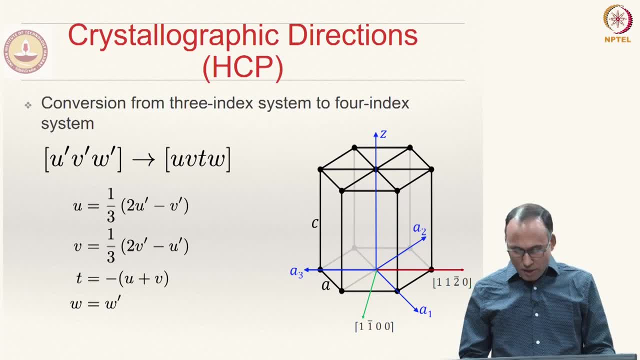 u, v, t are the projections along the z axis. So now, how do we actually? is there a possibility to convert from three axis notation to four axis notation? Let us say our three axis notation is represented by u, dash, v, dash, w dash. How do we go from this notation to? 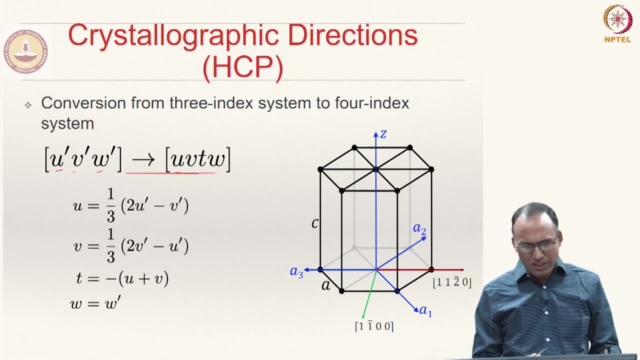 u, v, t, w. So this is one of the prescriptions, but there can be people can come up with different prescriptions if required. So one of this prescriptions is that the u in four index notation is related to the z axis. 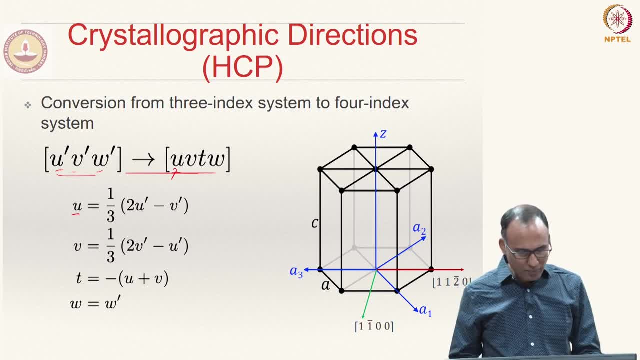 The three indices. notation as one-third 2 u prime minus v. prime v is one-third 2 v prime minus u prime and t is negative of u plus t. So that means the third index should also always be in a four index. notation should always be negative of sum of the first two. 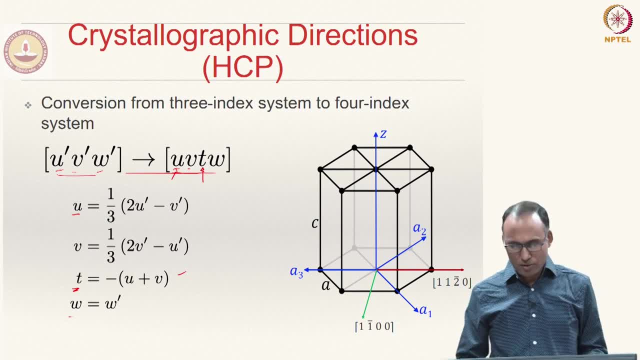 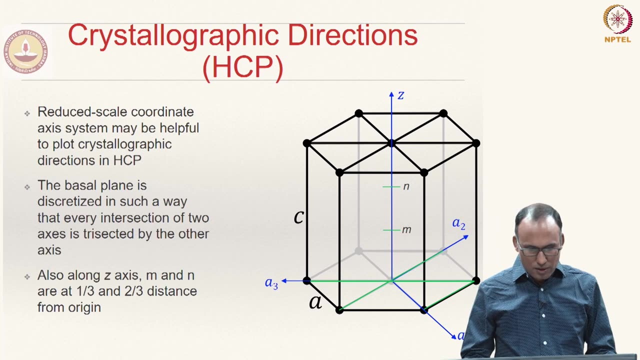 indices. that is important. and w is directly w prime. So this is how one can transform a three index notation to a four index notation. Once you do that, all the equivalent directions will are expected to be having z. So this is the third index notation. now we have to check the four analyses. This is 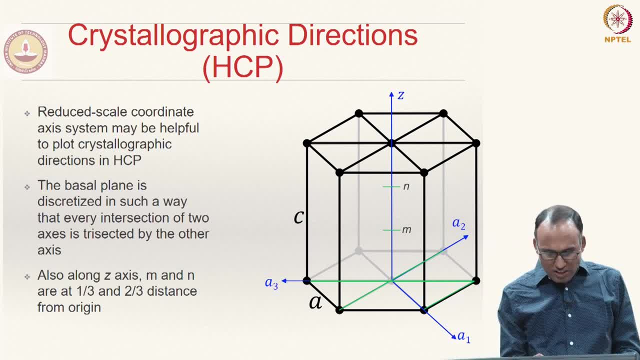 the third one. this is the fourth one. okay, So what we can do is we can basically get all these values and plus the value, plus the value of the four indices. So we are getting the three numbers: one, two, three, two, one, and so on. 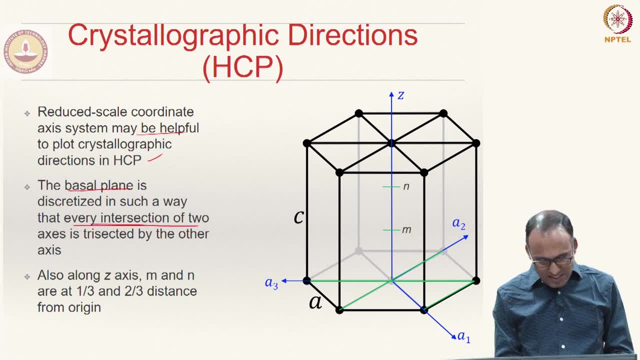 So in this equation we are going to solve the problem of two sets. One set is a few vertices, Okay, coordinate axis, and along the z axis also you trisect: m at m and n. m is at a distance one-third, z n is at two-third, m is at one-third, z n is at two-third and z. this point is one. 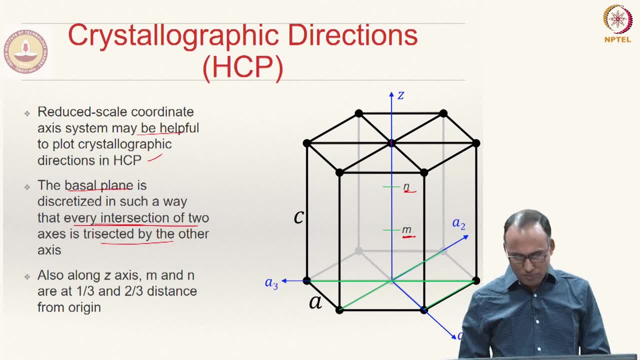 in the one-third of the lattice vector dimension there. So here, this is how we do the trisection. So this is the trisection of coordinate axis along A 2, and that is A 1 and A 3.. Now, if you have that, now we can actually see how. 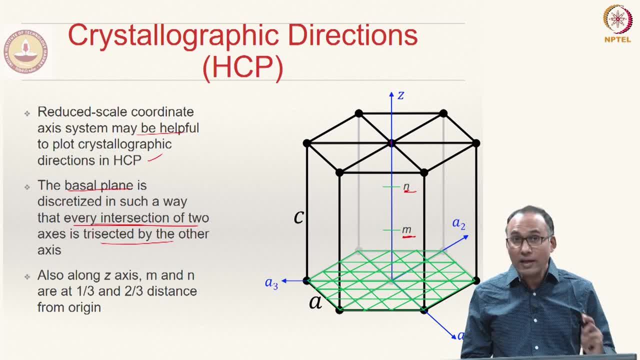 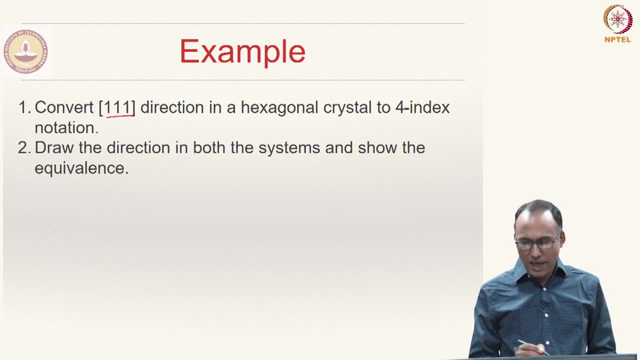 do we use this to represent the coordinate directions for hexagonal closed packed structure. So now let us see how do we convert 1, 1, 1 direction in a hexagonal crystal to four index notation and then draw the direction in both the systems and show the equivalence that 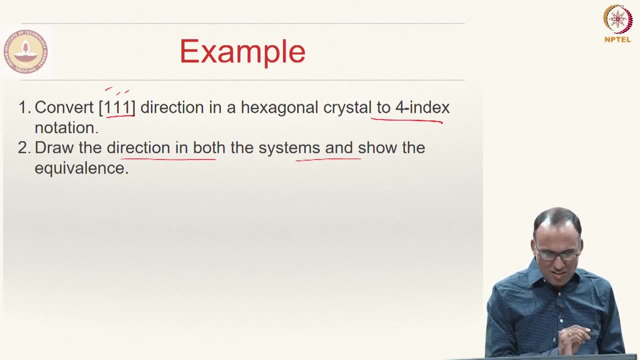 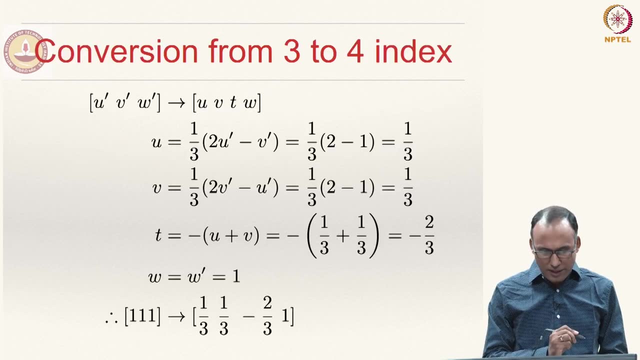 is the problem that we have to do. So this is u dash v dash t dash- sorry, u dash v dash w dash- and that you have to convert to u dash v dash t dash. You want to convert it into u v t w right, So that that the transformation from u dash. 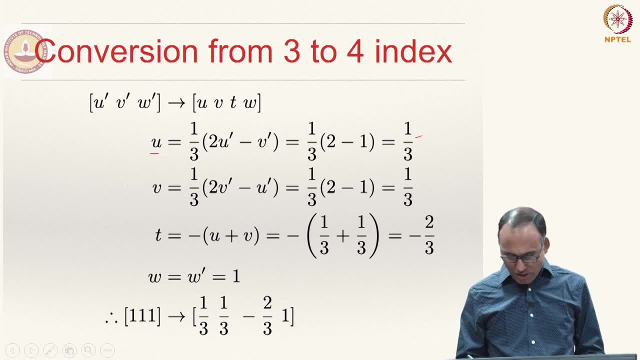 to u is given by this formula. So it will become one-third, one-third minus two-third and one, So one-third, one-third minus two-third and one. so that should be written as one-third, one-third, two-third, bar and one, But of course again, the minus should not be written as minus. 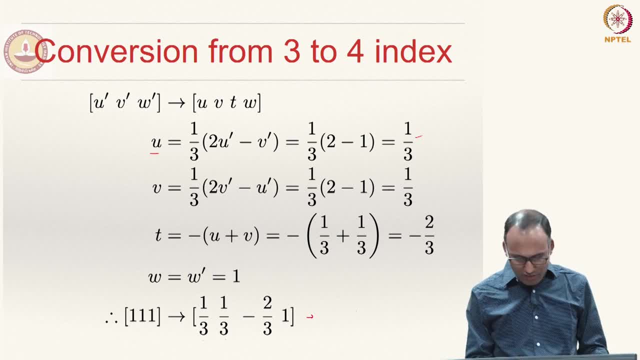 but you can see that minus of one-third plus one-third, Okay, 1 third. So it should always. the third one is: you really do not have to calculate t, you just have to calculate u and v. the t will be negative of some of these two And 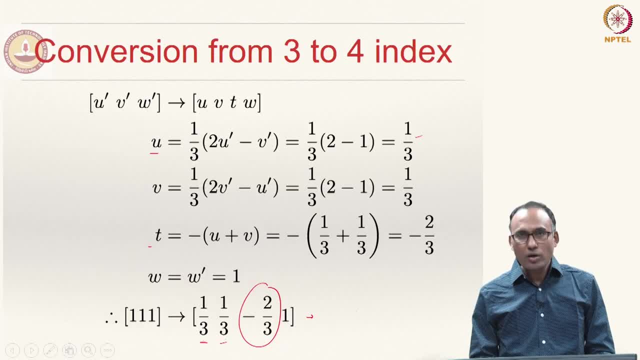 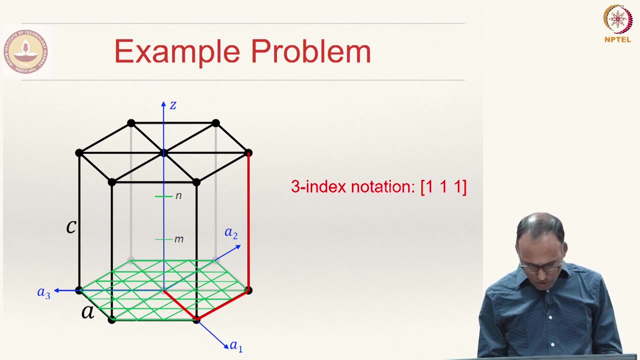 then you need to show that on the hexagonal crystal lattice, hexagonal unit cell. we let us show that. So this is 1 third distance. So we have to move 1 third along A, 1, that is your 3 index notation: 1, 1 and 1.. So that is our 3 index notation. 4 index notation. 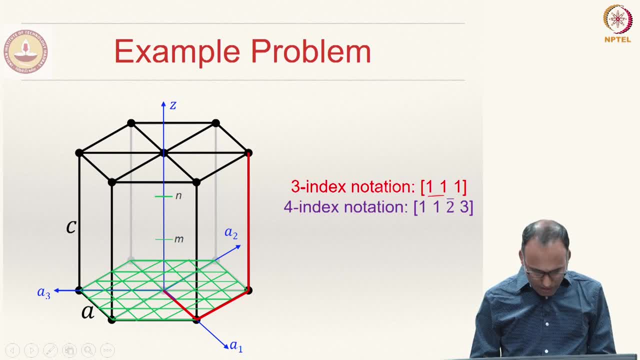 you have to move 1 third. So that means along A direction, So that means from there to there and so on. This is our 1 third along x axis. 1 third along A 2 axis, minus 2 third, because A 3 is shown in this direction. So minus 2 third is this, and then this is 1 unit. 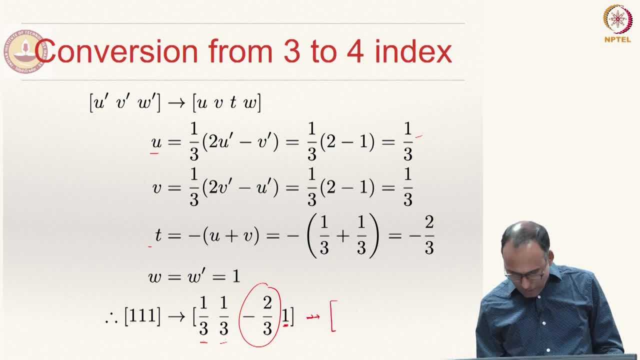 So, but the way to represent that is actually when we are representing coordinate, so the crystallographic directions. you do not work with this. fractions. you try to convert into smallest integer. So multiply everything with 3, that means 1, 1, 2 bar, 3.. Here 1 actually. 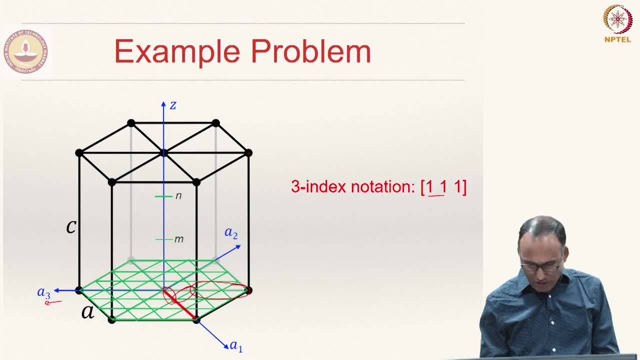 means 1 third distance on your crystallographic plane. So that is why your 1, 1, 2 bar 3 means 1, means 1 third, along that line in 4 index notation, Again 1 third and 2 times 1, 2, that is 2 third, and 3 means 1 third, 2 third and 3.. So that 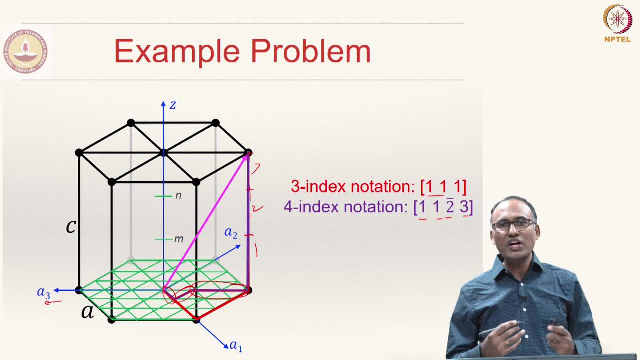 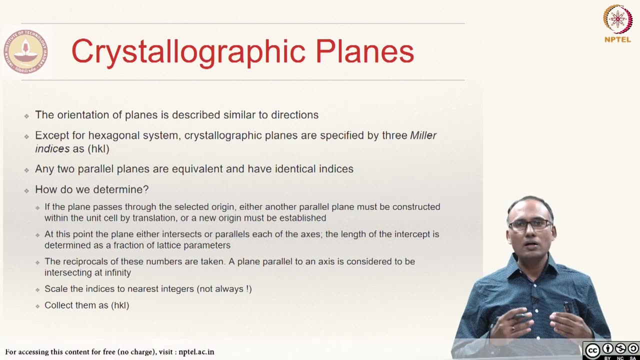 means this is 1, 2, 3.. So 1 third is 1 unit in when you are talking about 4 index notation and both of them are showing the same crystallographic direction. So, having discussed how do we represent the directions? 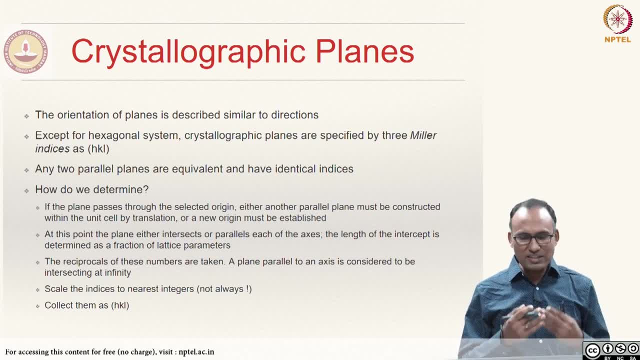 So only 2 parallel planes. so this is for 3 index notation. For 4 index notation you have to have h, k may be w, L, 4 index notation. We are going to discuss about 3 index notation and then 4 index notation. the same philosophy that we have used for directions can be applied. 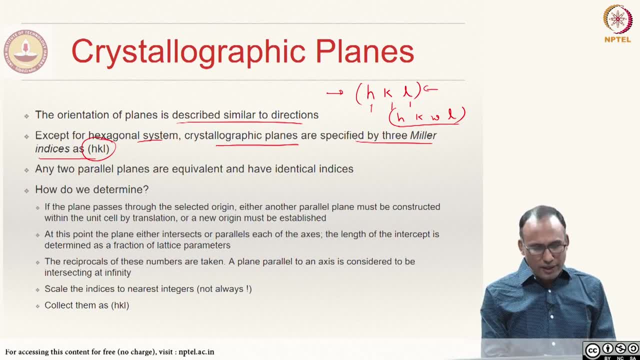 to planes as well And note that any 2 parallel planes are equivalent and has identical indices. So how do we determine these indices? Miller indices for crystallographic plane. Now, first let us we need to check if the plane is passing through the origin. You have a crystal cell. 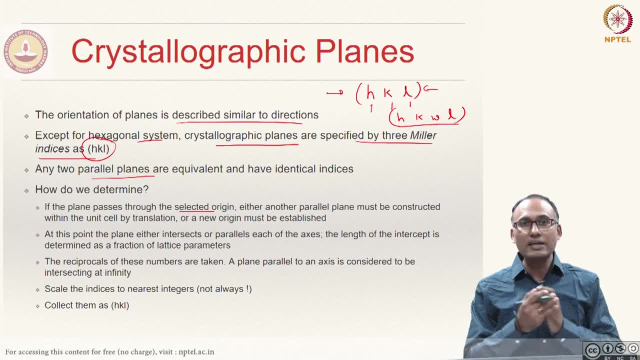 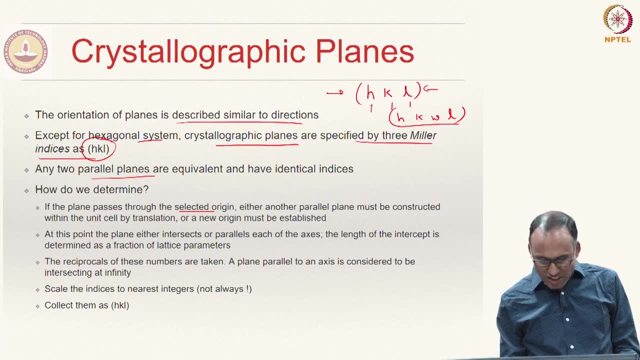 unit cell and you need to check the plane for which you want to write the Miller indices whether it is passing through the origin of the unit cell that you have chosen. So if the plane passes through the select origin, then what do you need to do? You need to either: 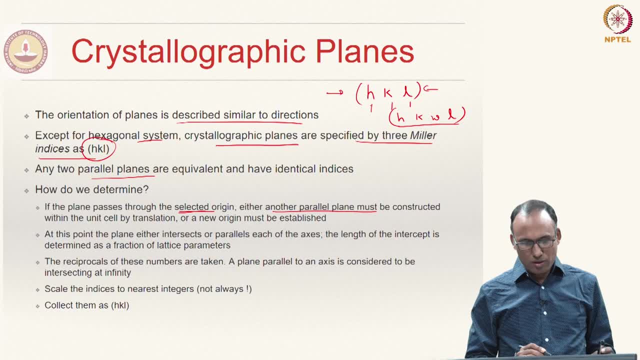 another parallel plane must be chosen within the unit cell. another parallel plane must be constructed within the unit cell by translation. or you change the origin, you have to choose a new origin. That means the basic guideline is that the plane should not be passing through. 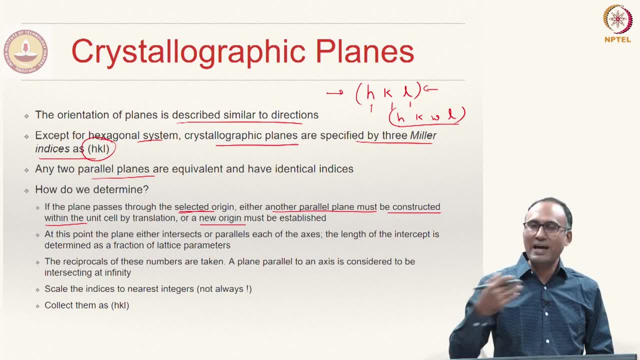 the origin, if at all the plane is passing through origin, because we said all parallel planes are parallel, Equivalent and have exactly same indices. you just have to translate the plane such that it is parallel to the original plane and then it is not moving, it is not passing. 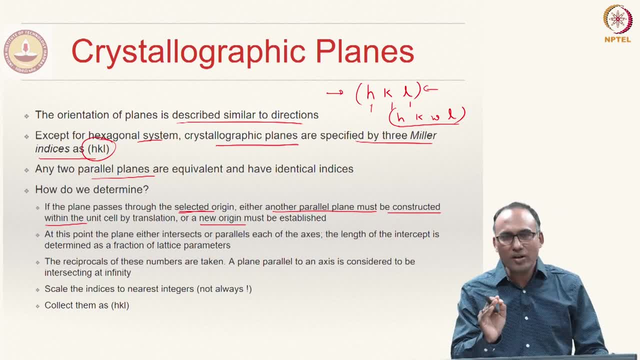 through the origin. All that we need to do is ensure that the plane is not passing through the origin. And at this point what happens? the plane is going to either intersect the coordinate axis or it will be parallel to the coordinate axis, because, if originally, 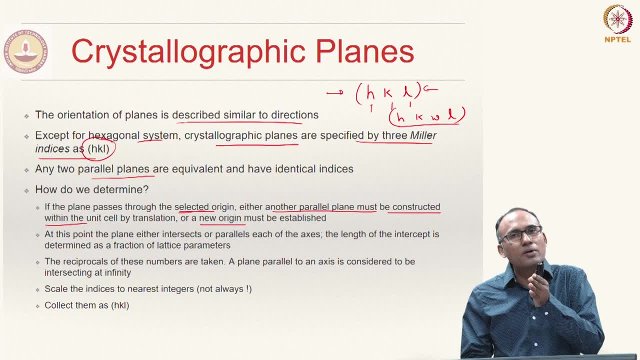 it. if it is parallel to one of the coordinate axis, by translation it will not become parallel, non parallel, it will still remain parallel to the coordinate axis. So at this position point of time, your plane should either intersect one of the axis or 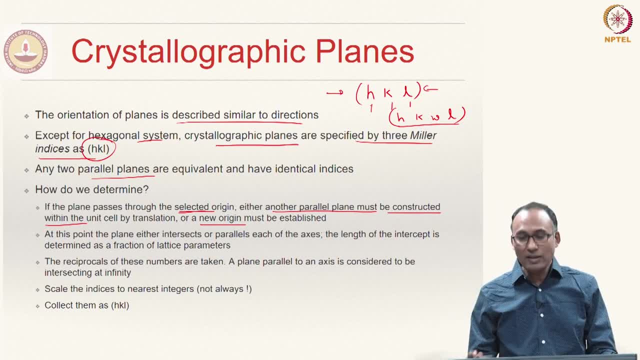 it is parallel to one of the coordinate axis, And the length of the intercept, if at all it is. you know the at what length it is intercepting. So the length of the intercept is determined as a fraction of the lattice parameter. You have to write the length of the intercept. 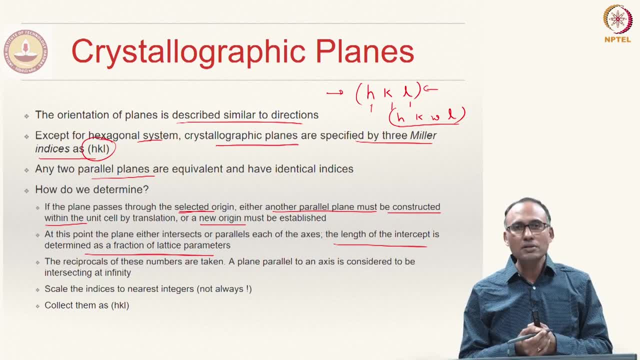 as a fraction of the lattice parameter, And then you have to take the reciprocals of those numbers. So first you have to identify the intercepts and write them as a fractions of the lattice parameter. So if it is intersecting, 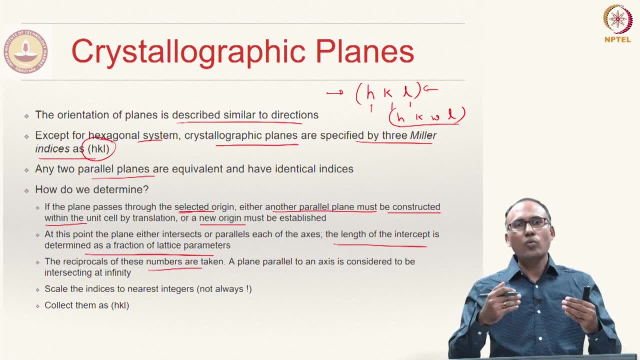 at the half the distance, then you have to write one half- a by 2,. if it is intercepting at a distance a by 2, then you have to write one half And then you take the reciprocals of them. So the reciprocals of the numbers are taken, and if a plane is parallel to x, 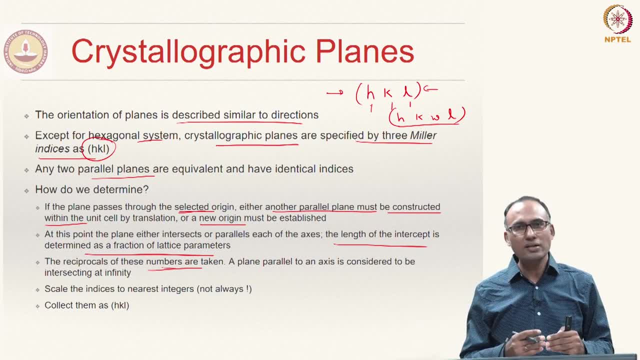 axis, that means it is intersecting x axis at infinity Right. If it is parallel, then the reciprocal of that will be 0. Right. So now, all the again, scale the indices to the nearest integers. Sometimes you do not actually do the scaling. 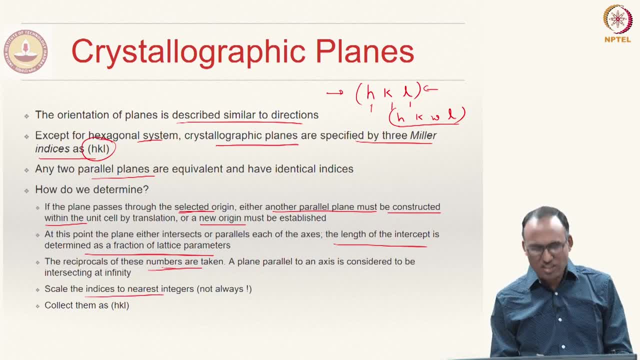 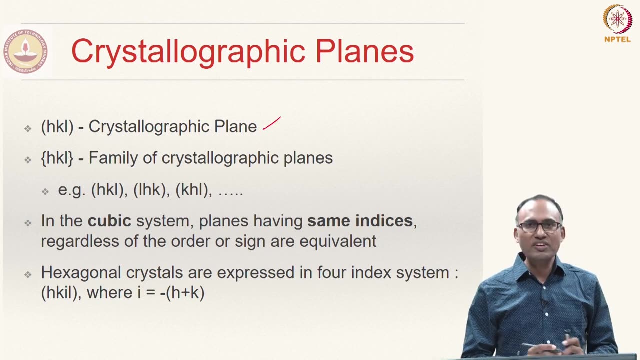 but usually in this class we will do the scaling- scaling to the nearest integers, and then collect the numbers and put them under parentheses. That is how you will identify crystallographic miller indices for crystallographic planes. So this is the definition representation. 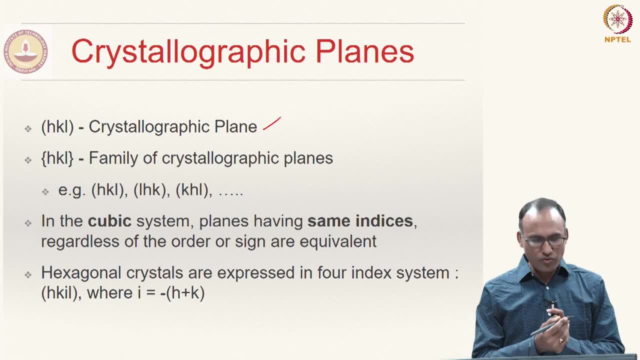 for crystallographic plane and the family of crystallographic planes are represented or designated with curly braces In a cubic system. if you are looking at cubic system, the planes having same indices, regardless of the order or sign, are equivalent for cubic material cubic systems. They need not be parallel but they can be equivalent planes. 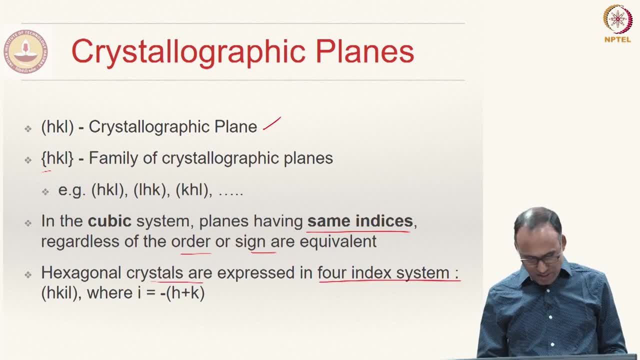 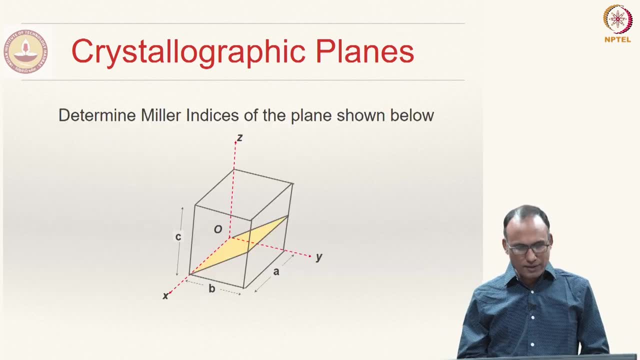 And hexagonal crystals. Right And hexagonal crystals are expressed in four index system wherein they are represented: h, k, i, l, where i is equal to negative of h plus k. All right, So now let us look at this particular system and let us try to see whether we can. 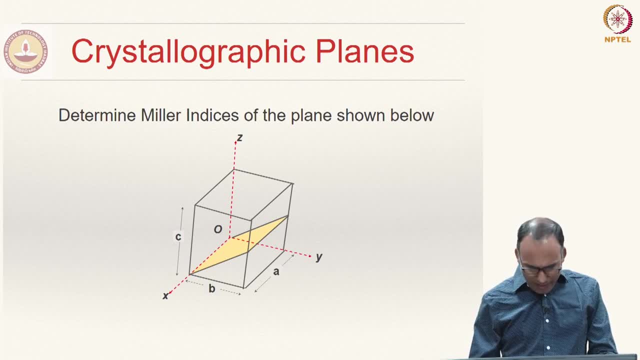 identify the miller indices for this plane, You can see that this plane is actually passing through the origin. This is our origin. It is actually passing through the origin. So the first check to be made is to see whether the plane is passing through the origin. If 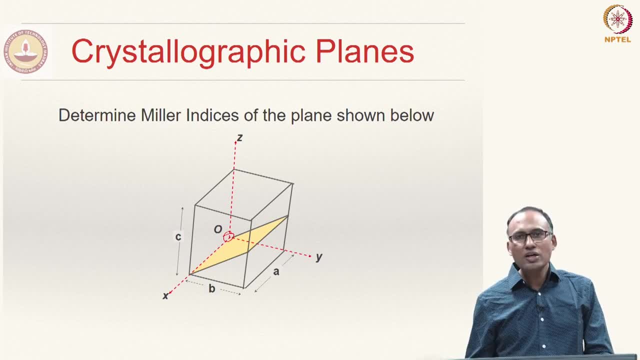 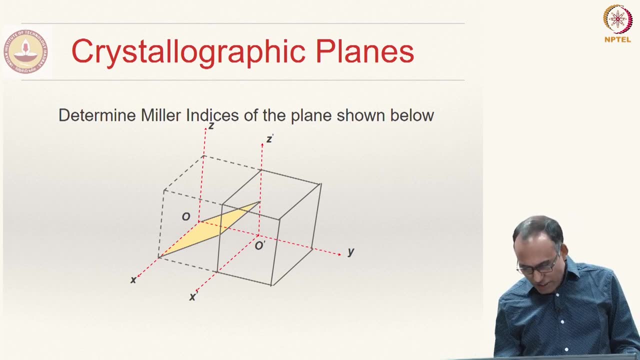 the plane is passing through the origin. what is that we need to do? Either change the origin or move the plane, translate the plane. So what we have done is we have actually changed it. So initially here, now we have moved our coordinate system. 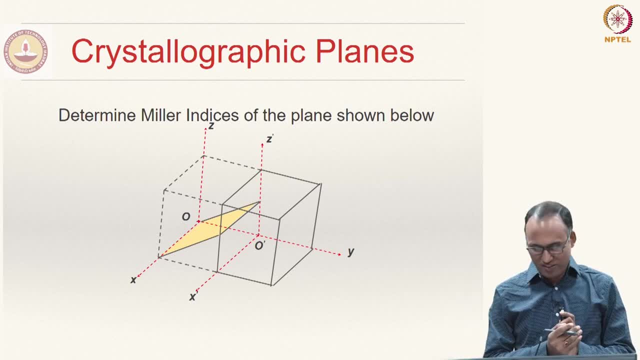 from this point to this point. So that means you have moved the origin, but keeping the plane the same. So now, o dash is your origin and x dash, y, z dash is our new coordinate system. Now the plane is not passing through origin. Now let us look at where this plane 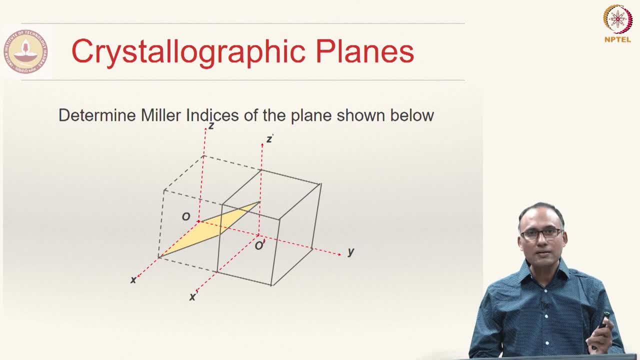 is intersecting? It is intersecting x axis, y axis and z axis. Is this plane intersecting x axis anywhere? It is actually parallel to x axis, So it is not intersecting x axis. Where is this intersecting y axis? So this is intersecting y axis at this point, So that means negative. 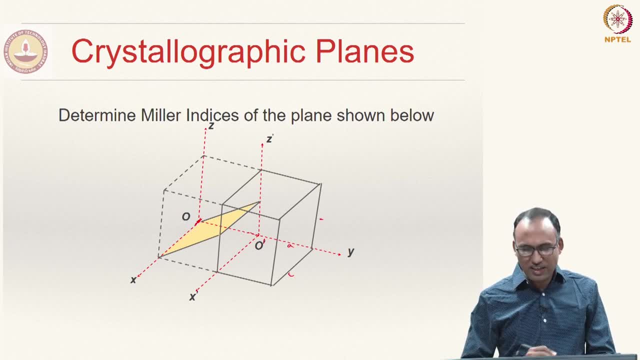 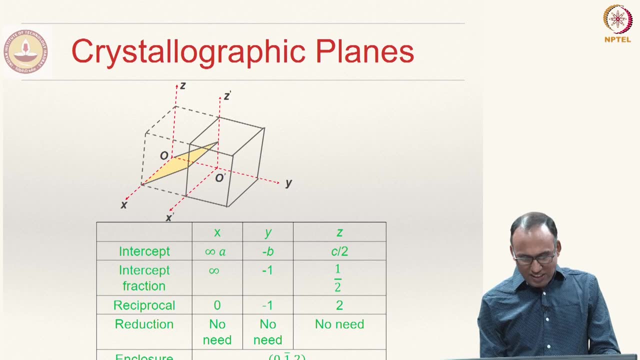 a. So let us say this is a, a, a. It is intersecting at negative a and z axis. it is intersecting at positive a by 2. Right, So x intercept is in parallel. That is why infinity times a and y axis it is intersecting at minus b and z axis. it. 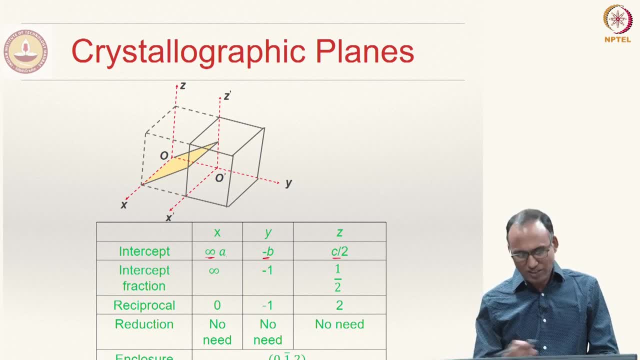 is intercepting at c by 2.. a, b, c are your lattice parameters, for instance, And then you write that intercept as a fraction of your lattice parameters. So that is why I am writing infinity minus 1 and plus half, And then you need to take the reciprocals. 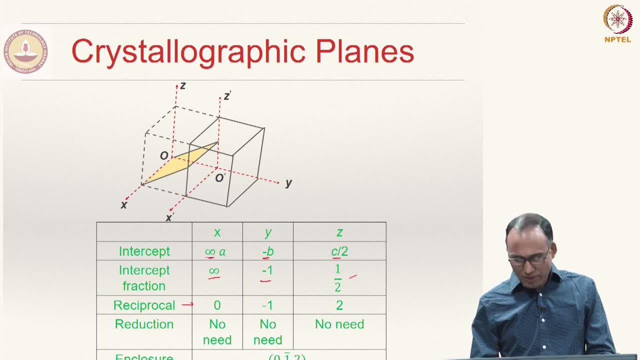 Reciprocals of them 0, minus 1, 2.. Do we need to do any reduction? Because there are no fractions, So there is no need for reduction And hence the enclosure will be 0,, 1 bar and 2.. So that is the representation of that plane. 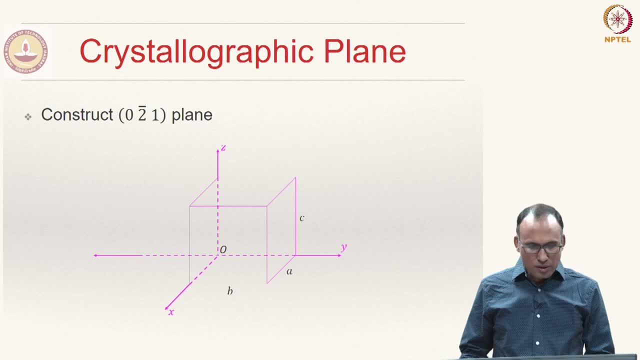 And now let us construct another plane: 0, 2 bar 1.. So, in order to construct, what we need to do is, first, we need to find the intercepts. Where are, what are the intercepts? Intercepts. 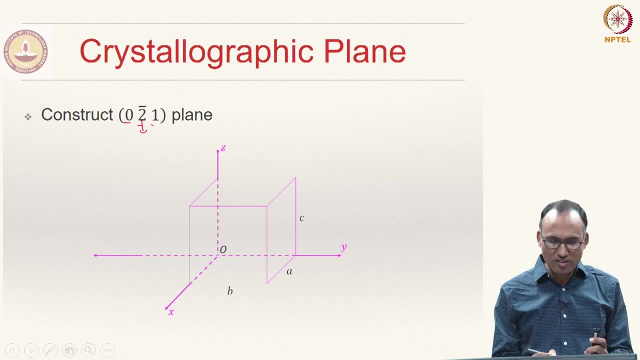 will be the reciprocals of them. Right. When we are constructing, we have taken the intercepts Right And then taken the reciprocals of them to represent the mirror lattices. Now, in order to find the intercept, you need to find the reciprocals. So that is infinity minus 1. 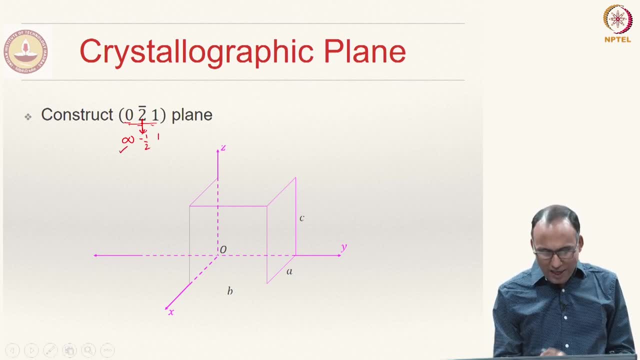 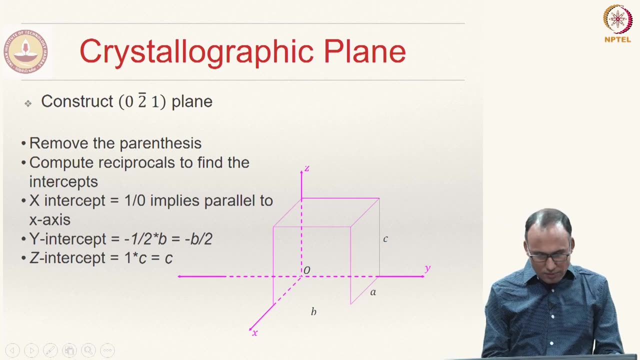 by 2, 1.. That means this plane is going to be parallel to x axis, going to intersect y axis at minus half and z axis at 1.. Right, So implies parallel to x axis, y axis at minus half, z axis at 1.. 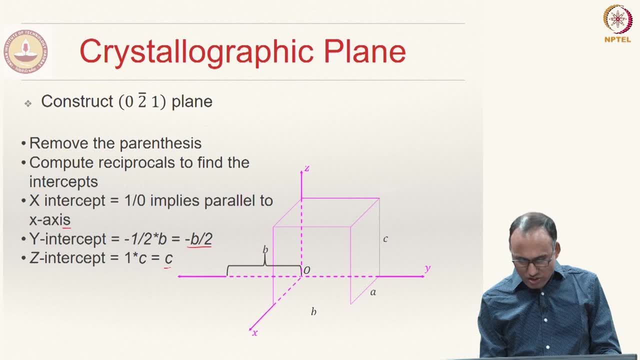 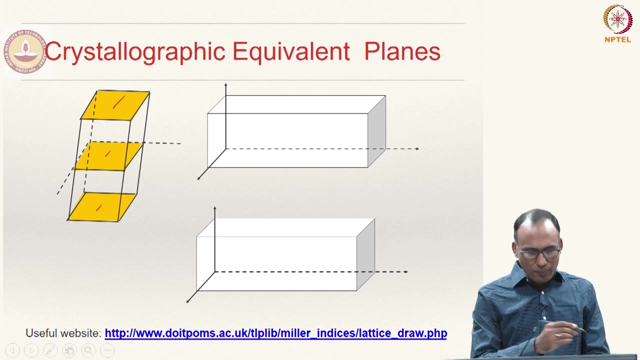 So that is. So this is b, So this should be intersecting y axis at minus half and z axis at 1.. So that is our plane: 0, 2 bar 1.. So equivalent plane. so this is all. parallel planes are equivalent. 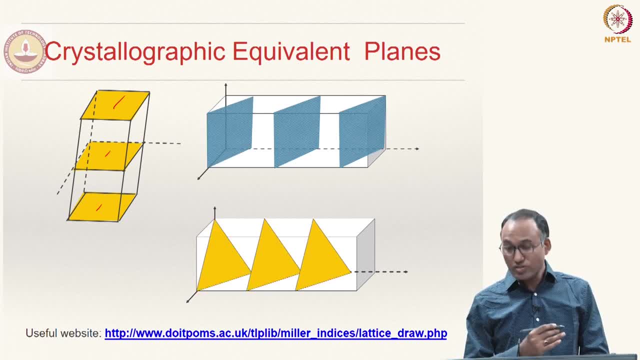 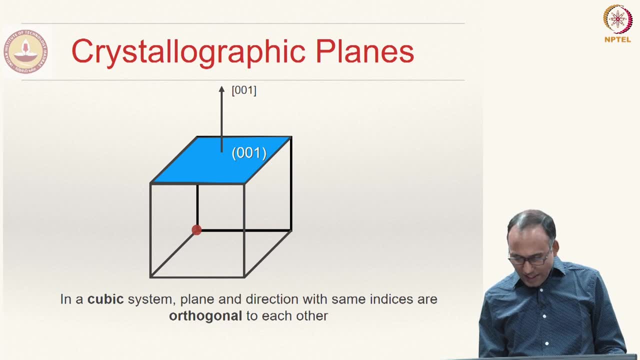 So that is also equivalent: all parallel planes and they will have same set of indices. And in a cubic system, for instance, a plane and a direction with same indices are orthogonal to each other. That means in a cubic system, for instance, a plane and a direction with 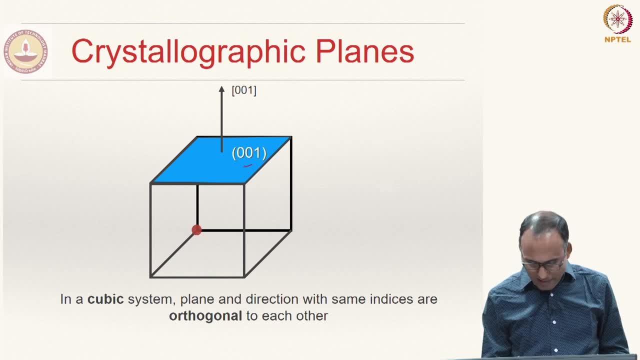 same indices are orthogonal to each other. That means, if you take a plane, 0,, 0,, 1, because this plane is intersecting z axis at 1,, but it is parallel to x and y axis. So that is. 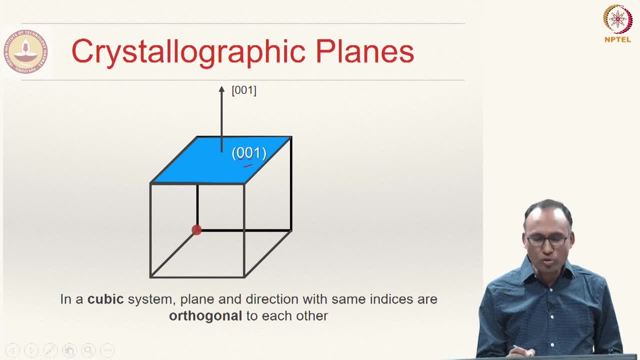 why these indices are 0,, 0,, 1.. And the normal to this plane, the direction, crystallographic direction that is actually normal to the plane, will have exactly the same indices as the indices of the plane itself. But so the normal direction should be shown with a different. 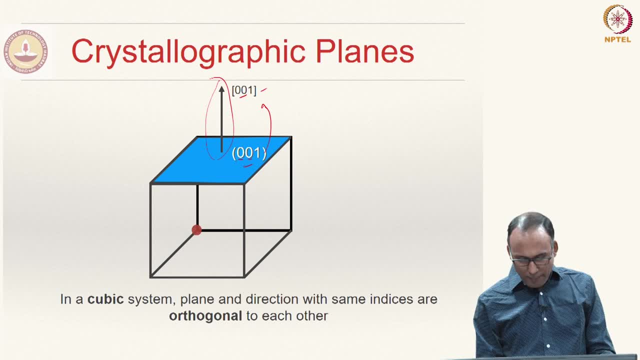 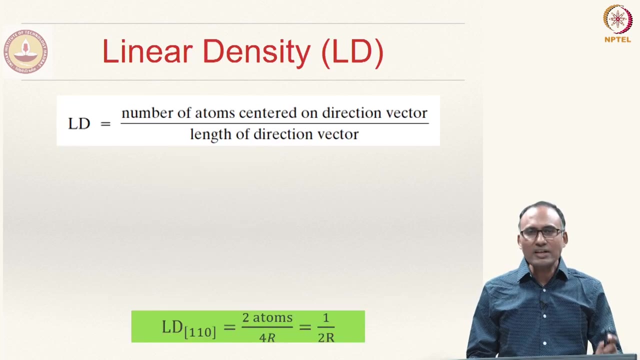 brackets. So in a cubic system, plane and direction with the same indices are orthogonal to each other. That is what orthogonal means to a plane, if something, a direction, is orthogonal, that is what is called normal to the plane. So now let us define something called linear density. What do we mean by linear density? 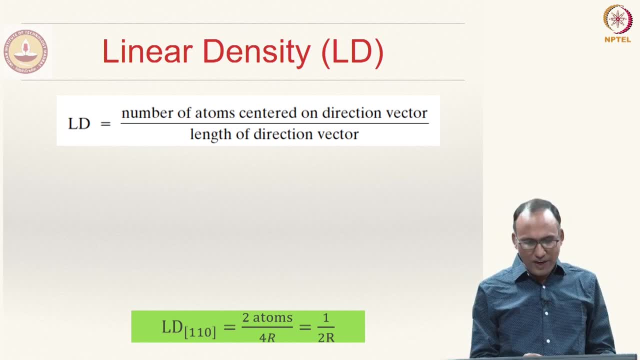 So the linear density is defined as the number of atoms centered on a direction vector. So we have defined a crystallographic direction. So on that direction vector how many number of atoms are centered, divided by the length of the direction vector, That is what is called. 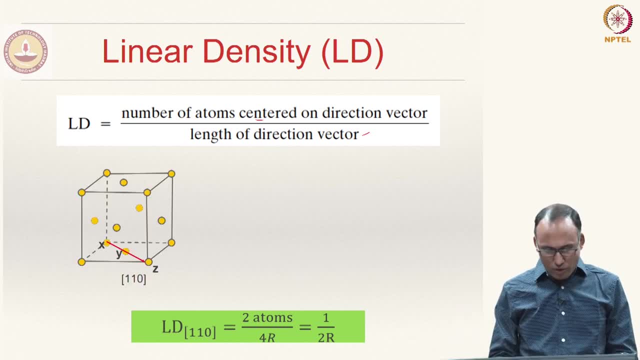 linear density. So if you take a 110, if you take a FCC material, then you have 110 direction. is this? How many atoms are there on 110?? There is one full atom and this atom is part of another atom. So this atom is another unit cell. This atom is also part. 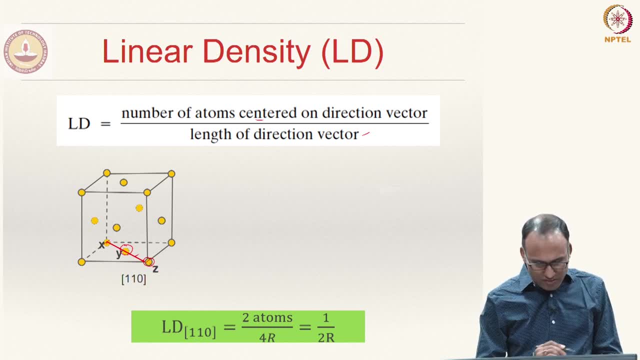 of another unit cell. So half of this guy is present here and half of this guy is present here. Effectively, you have two atoms lying on that direction, So two atoms divided by the total length. If it is r, then these phase centered atoms are in. these atoms are touching. 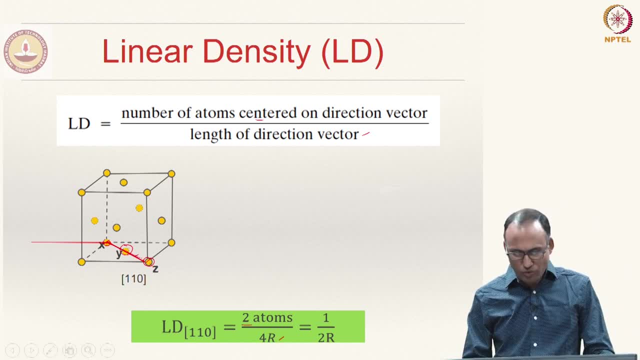 each other. So this will be 2 r and this is 2 r, So that total length is 4 r. So the linear density is 2 atoms by 4 r. So that means 2 by 1, 4 r, That is 1 by 2 r. So 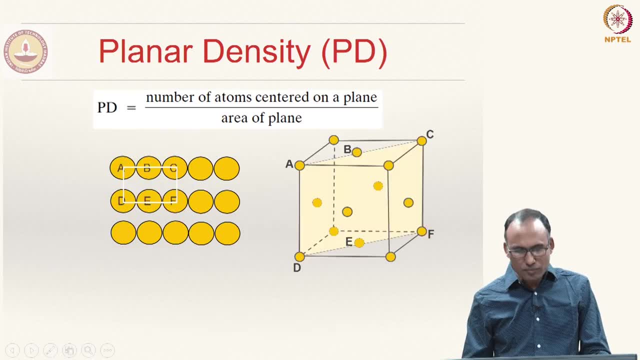 that is how, if you look at, that is how this looks like. So that is about linear density. Now, where we have defined a crystallography. So what we have defined, the crystallography, is the number of atoms that are centered on. 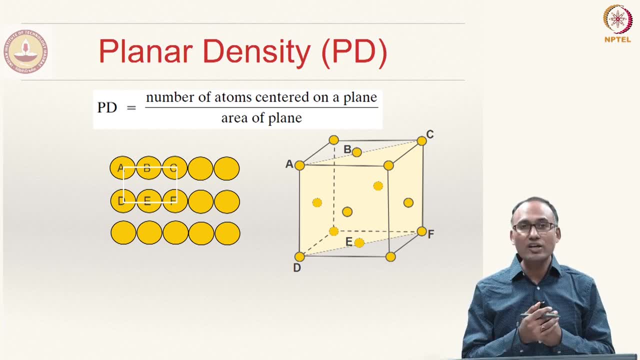 a plane divided by the area of the plane. So when we have defined a crystallography, then we can define the number of atoms that are centered on a plane divided by the area of the plane. So if you take this particular plane, what is this plane? by the way, It is? 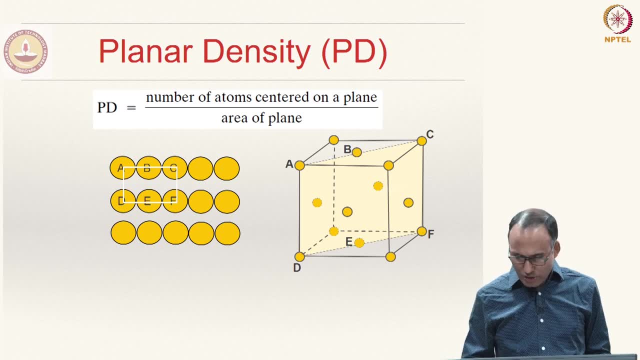 intersecting x axis at 1, y axis at 1 and parallel to z axis, and hence this should be 110.. This is what you call 110 plane in an FCC material, phase centered cubic structure material. And then let us look at the planar density. So this is how the atoms are arranged, and 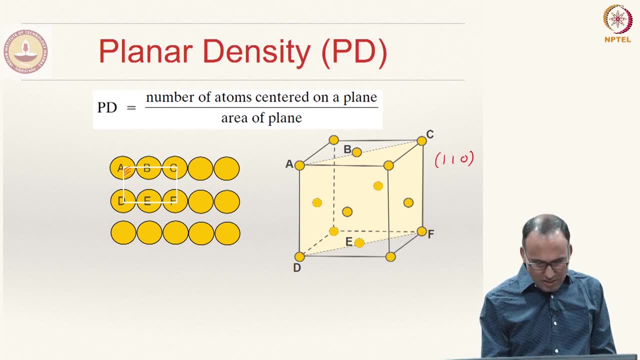 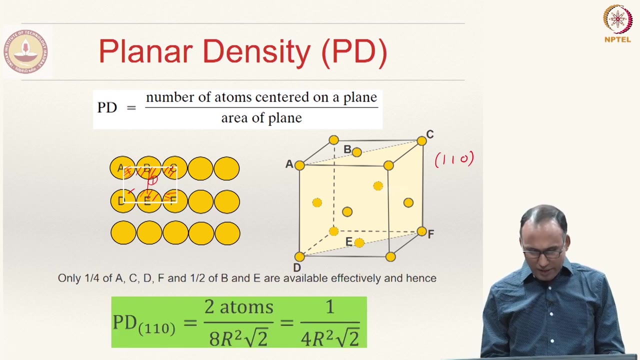 you can see that in this plane, this atom is, this part of the atom is available, this part of the atom is available, this part and that part, So effectively, these two together, one atom, these four together, another atom. right, So there are effectively two atoms available. 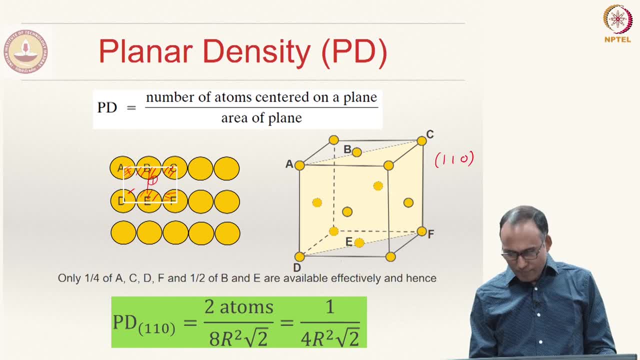 divided by the area of the plane. So you know. if this is a, you can find out the relation between. So what is this distance? this distance is 4 r, right? yeah, So this distance is 4 r and you need to find out this area, and that means this is a, this is a, So you can find. 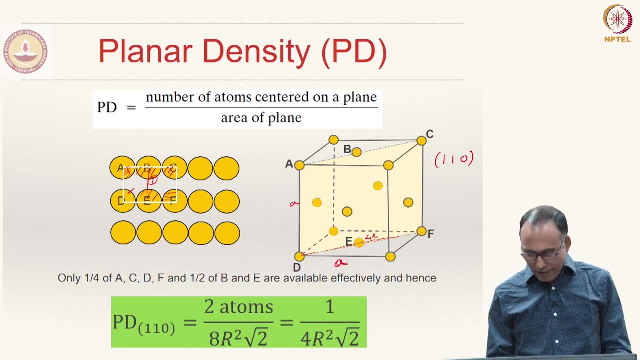 out what is the value of a and then that will actually be. the area will be 8 r square under root 2.. So the planar density of 1 to the power of 110 plane for FCC is 1 by 4 r square root, 4 root 2 r square. So the knowledge about 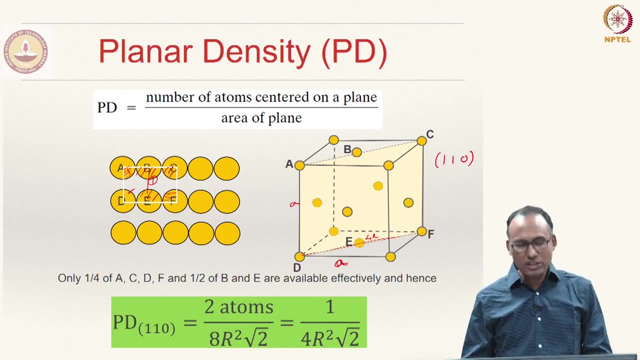 this linear density and planar density is a one of the important aspects to be known, because the planar density and linear density are going to give us some information about the deformation mechanism when we are talking about plastic, deformation in materials- And hence it is extremely important to know what are the planes in a given crystal structure. 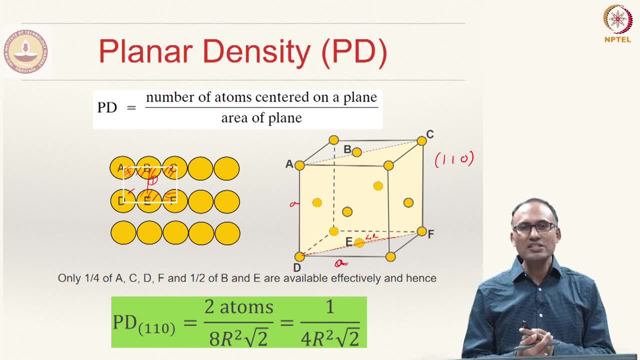 or a given unit cell which are most densely packed. that means which are having highest planar density or lowest planar density. What is the direction in which you have maximum linear density? that means that is the most closely packed direction. So it is important.